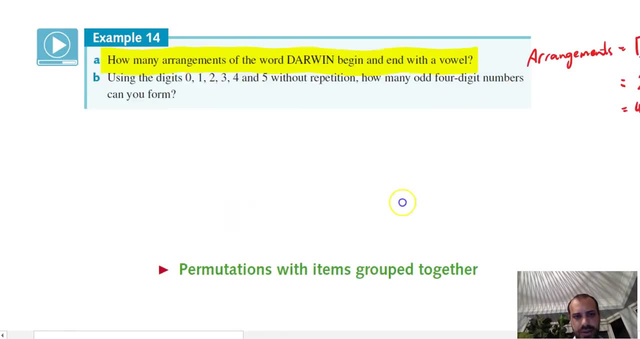 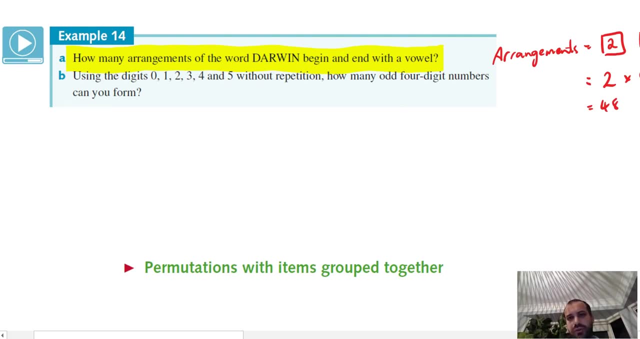 I get an answer there of 48.. All right, let's look at our next question here. Using the digits zero, one, two, three, four and five, without repetition, how many odd four-digit numbers can you form? All right, so they have to be odd. 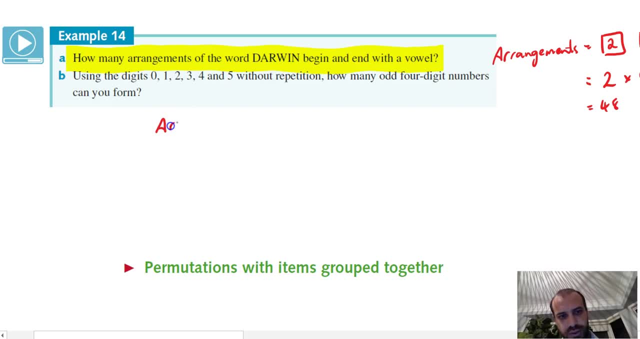 so in order for them to be odd, let's do a little box method again. All right, so first of all they're four-digit numbers. Maybe I'll use like a line method instead of a box. Now, how many odd four-digit numbers. So the last digit there needs to be a one, a three. 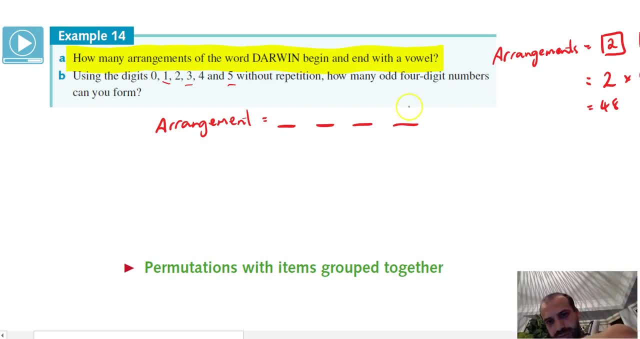 or a five. So there's three options for that one, And now we need to consider the rest of these. So there's one, two, three, four, five, six digits in total. So I would, at first glance, I would think that you can write the number five in here as sort of this: five options there. 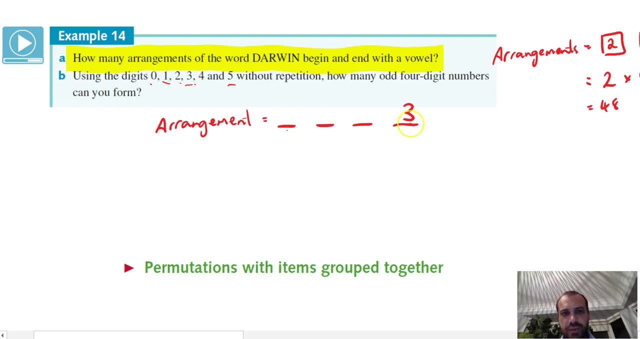 but I don't think it can. It can be zero and one of these odd numbers is sitting there, All right. so now that I know that one of the odd numbers is sitting there and this digit can't be zero, there are only one, two. 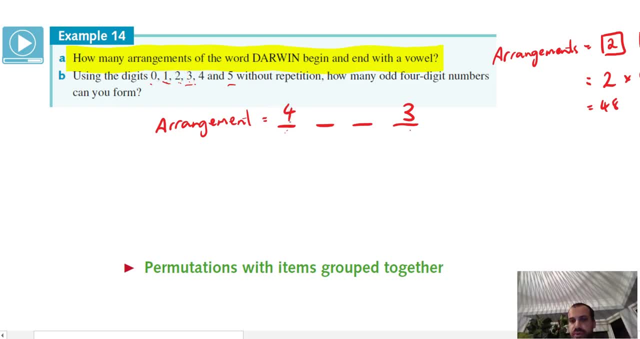 three, four options available to me at that specific point. So I've used up two of my numbers here. I can use any of the rest for the other two. So there were six digits in total. I've used two so I can have four here, And then I've used three now. 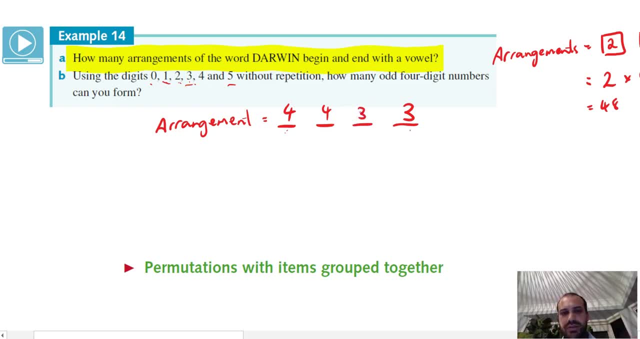 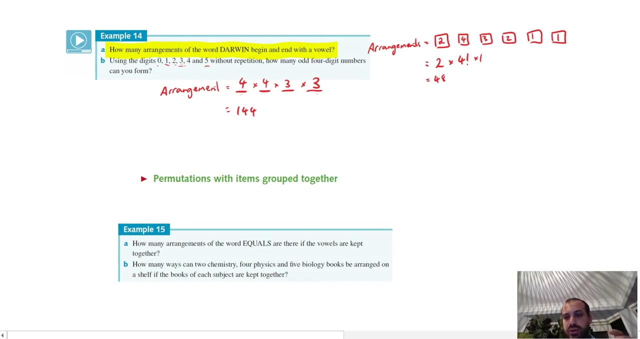 Six, so I can have three different ones there. So I say the answer is four times four times three times three, which is equal to 144.. All right, so those are some restrictions. Let's look at ones where the items are grouped together, where Bob and Jill need to sit in a rowing boat next to each. 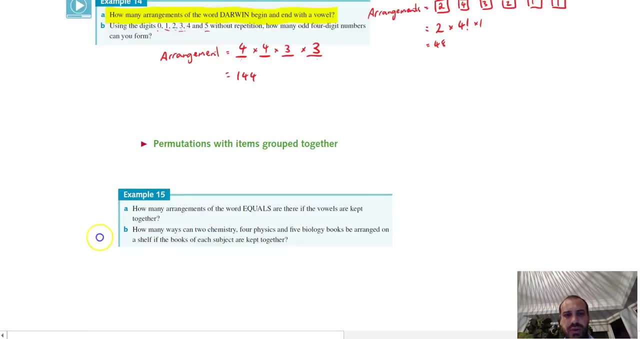 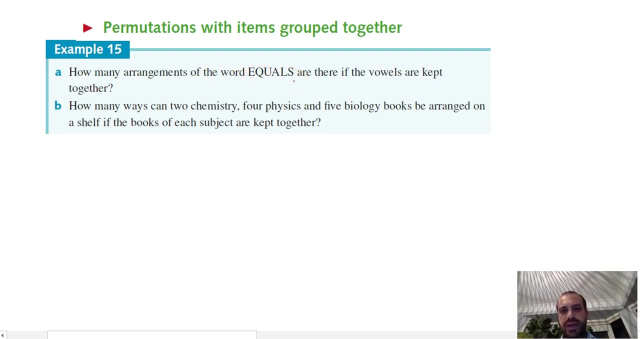 other. That seemed to be a classic one. Let's see what questions we've got here that are similar. All right, How many arrangements of the word equals are there if the vowels are kept together? Okay, so these are sort of a bit tricky, but the way to think about it is to think about the word. 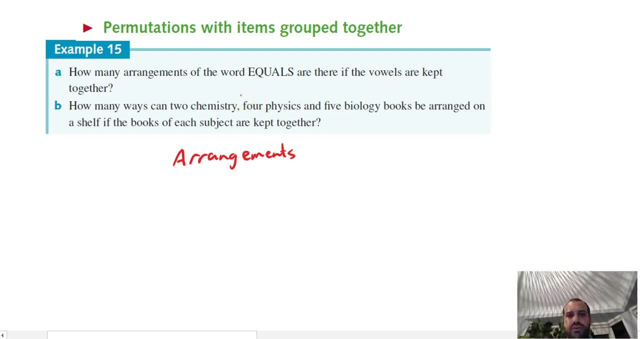 equals The three that are going to get grouped together: the E, the U and the A are going to get grouped together, So E U A becomes like its own letter all to itself. So now I have it's going to be equal to, so I'll just do E U A there. So that means that there's one letter. 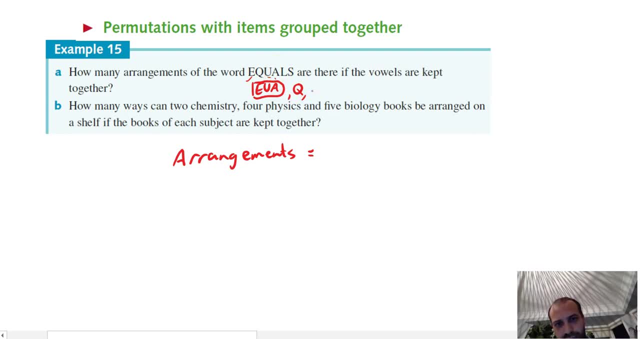 E, U, A, there's another letter Q, there's another letter L and there's another letter S, And if I'm going to arrange four letters that's going to be four factorial. So that's the arrangement of four letters, But one of the letters can be arranged. 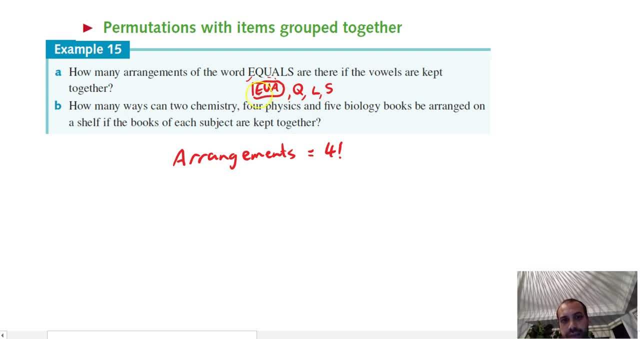 in multiple ways: E U A could be E U A, It could be E A U, It could be A U, E A, E U. It can be arranged in three factorial ways, because there's three items and I'm going to arrange all. 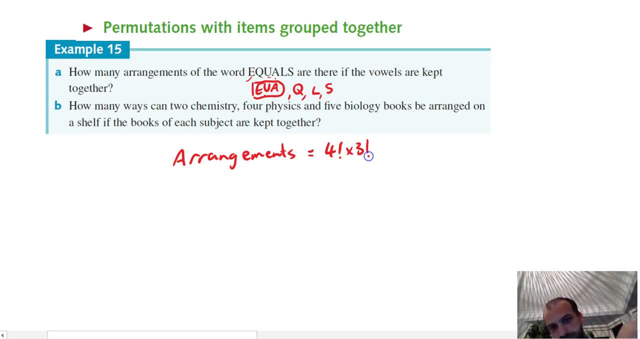 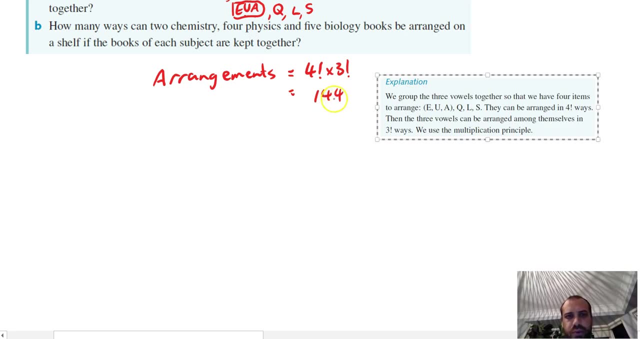 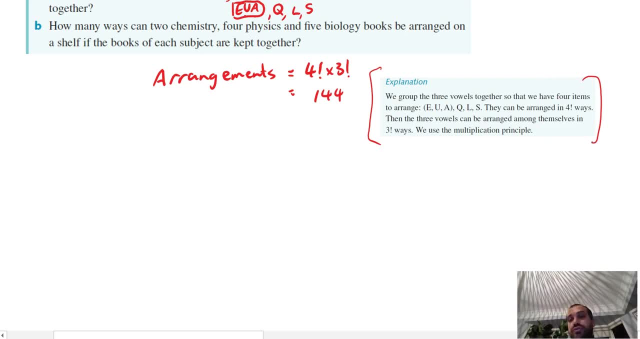 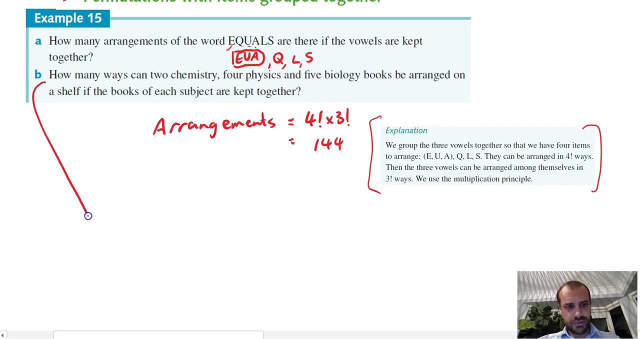 a little textbook explanation of how they've described how they do that sort of question as well. So if I didn't make a lot of sense there, you can. you can read through that one as well. This next question here really kicks it up a notch. It says: how many ways can two chemistry 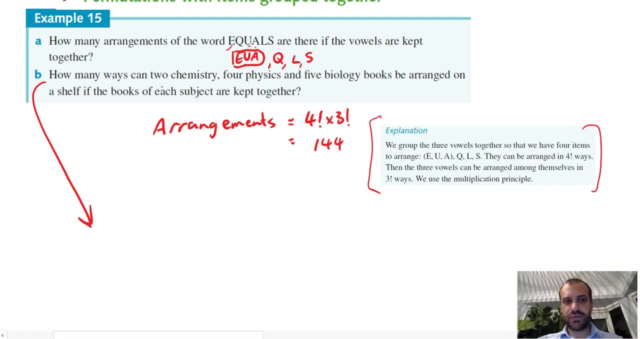 four physics and five biology books be arranged on a shelf if the books of each subject are kept together. So let's look at the books. First of all, two chemistry books, there's four physics books and there's five biology books, And I've put them in their little 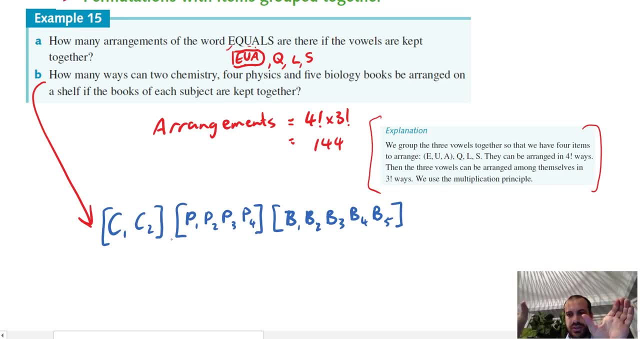 brackets here, because I'm treating them as a single units, right? So the way that. so I've got three objects there, So the way to arrange three objects is just two, three factorial sorry, which is six. So let's, let's write in our arrangements: arrangements is equal to. So the ways to do these.